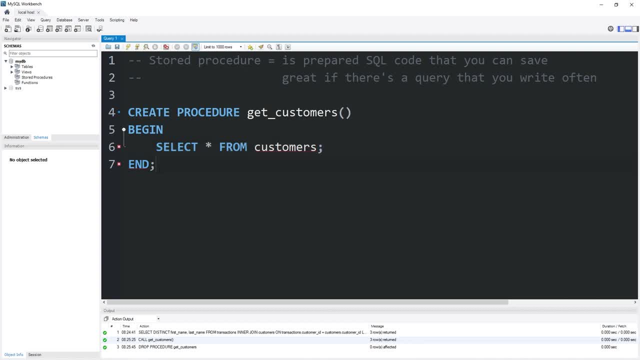 at this semicolon. here We end all statements with a semicolon rather than at the end. Our semicolon is known as a delimiter. It's kind of like the period at the end of a sentence. We're telling mysql that our statement ends here, but we need our statement to end here, after the. 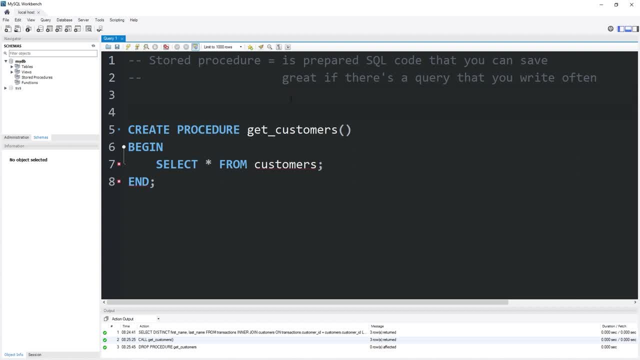 end keyword. We can actually change the delimiter temporarily: Type delimiter- before we create the procedure: Type delimiter before we create the procedure. Type delimiter before we create the procedure. Typically, when people change their delimiter temporarily, they'll either use two forward slashes or two dollar signs. I'll stick with the dollar signs because I think that's cooler. 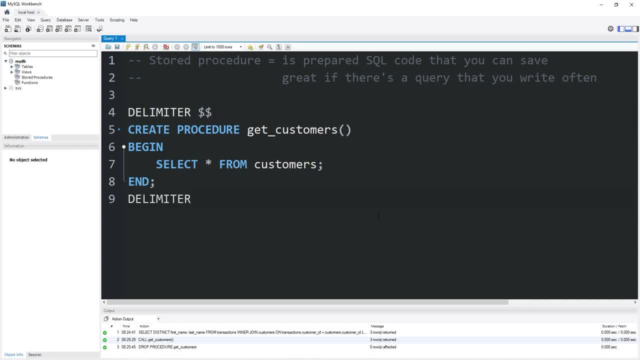 After we create our procedure, let's change our delimiter back to the semicolon. Mysql no longer recognizes our semicolon as the delimiter After the end keyword. I will use our new delimiter to end the statement. That should work. now Let's execute the statement. 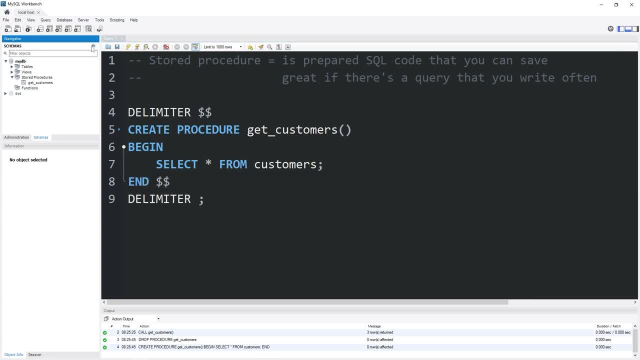 We have created our procedure. I'm going to refresh my navigator window. Underneath stored procedures, we have our stored procedure of getCustomers. To invoke the stored procedure type, call the name of the procedure: getCustomers. add a set of parentheses, then a semicolon. That will execute whatever code you stored within your 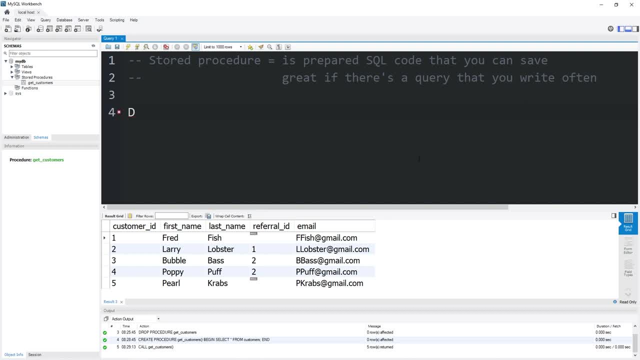 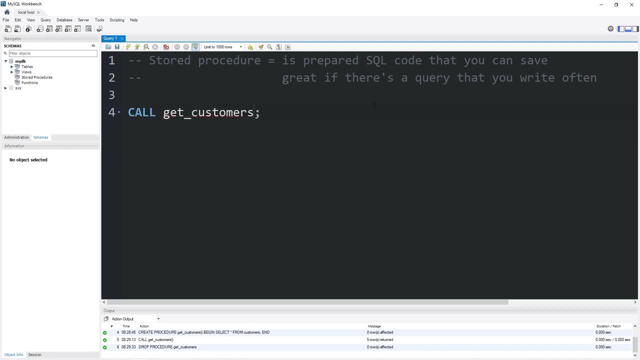 stored procedure. To drop a stored procedure, you would type: drop procedure. the name of the procedure: GetCustomers. Let's try another example. This time we will send our procedure a piece of data, within the set of parentheses, a customer ID number, such as 1,, 2,, 3,, 4, so on and so forth. 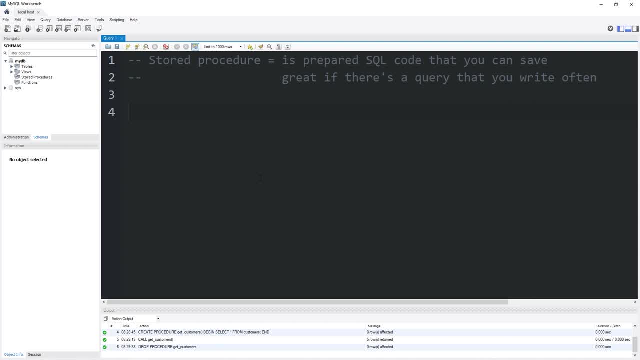 We will get a customer by their customer ID. We will create a procedure. I will name this procedure findCustomer. Add a set of parentheses, then a semicolon That will execute whatever code you stored within your procedure To find a customer by their customer ID when we invoke the stored procedure. 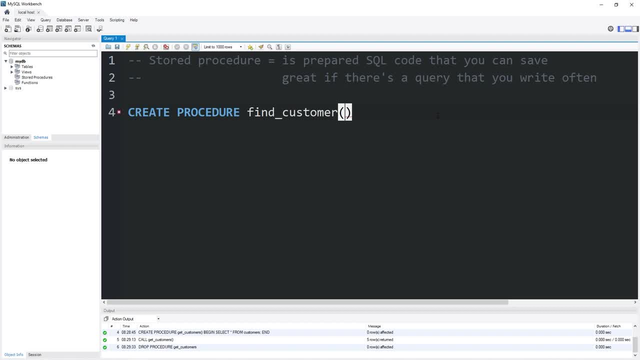 within the set of parentheses we will need to place a customer ID, But when we create the stored procedure, we have to set up what is called a parameter. We will type in then a nickname for that piece of data We're passing in a transaction ID. 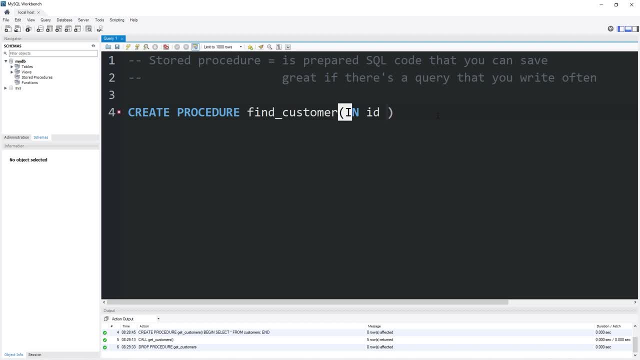 I'll give this parameter a nickname of ID. Then we need the data type of what we're passing in. We're passing in an integer, So we have one parameter set up. Let's use that begin keyword, that end keyword, list our statement or statements. between these two keywords, I will select all from my 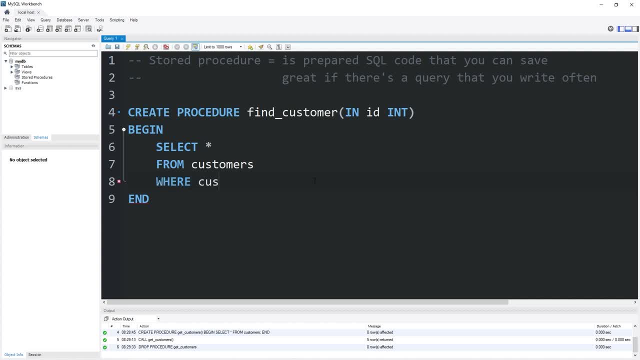 customers table where my customer ID equals the ID that we pass in that nickname. We need to change the delimiter because my SQL machine is not working. We need to change the delimiter because my SQL machine is not working. sql thinks we're trying to end our statement here, but we need it to end after the end keyword. so 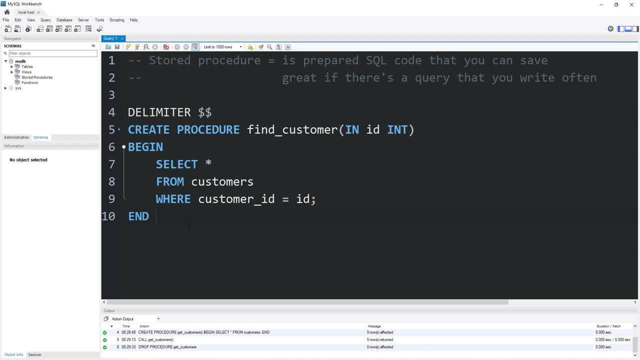 let's change the delimiter to double dollar signs, then change it back. all right, we have created that stored procedure. let's invoke it. call: find customer. within the set of parentheses, we need to pass in a customer id number. let's pass in one that would give us fred fish. two is larry lobster. 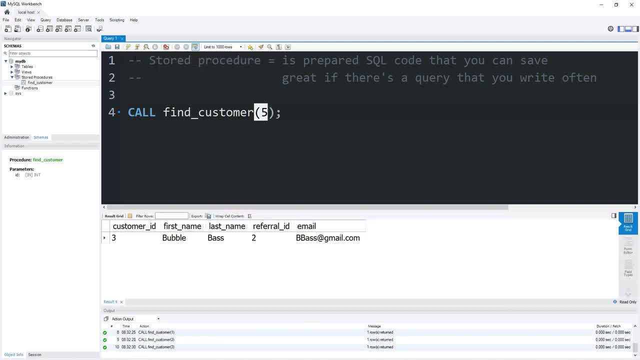 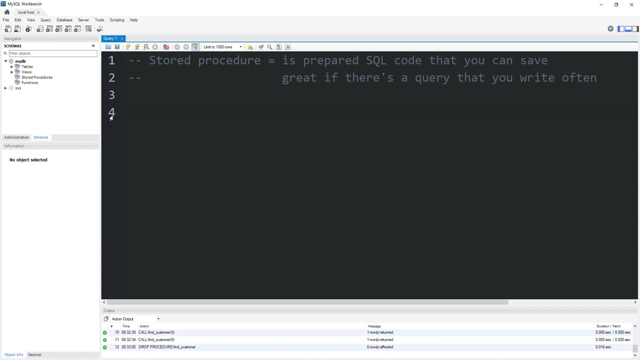 three is bubble bass. five is pearl crabs. when you invoke a stored procedure, you can pass in some data depending on what you need exactly for your stored procedure. let's drop this procedure. then do one last example. drop procedure: find customer customer, customer customer customer. this time we will send two arguments, two pieces of data, a first name and a last name. 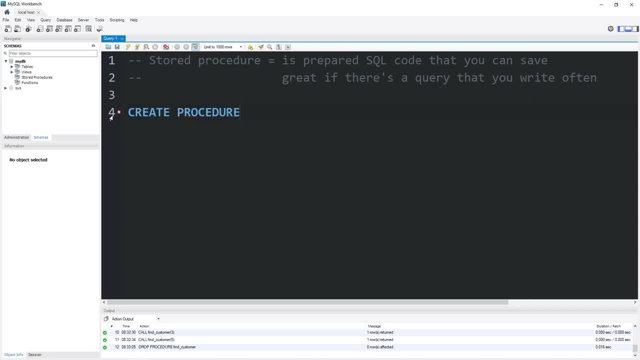 create procedure- find customer. within our set of parentheses, the first piece of data we'll pass in will be a first name, but first is already a keyword, maybe f name, meaning first name. then the data type. let's see for customers, the data type of first and last names is varchar50- varchar50.